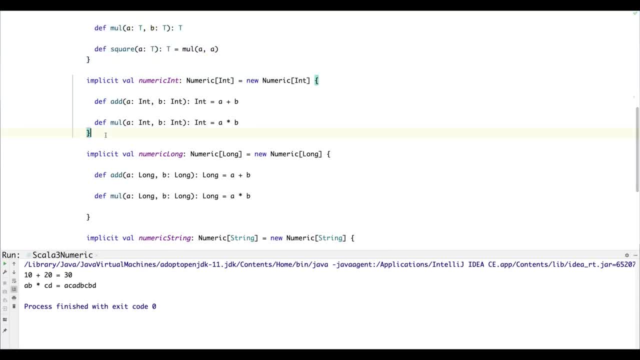 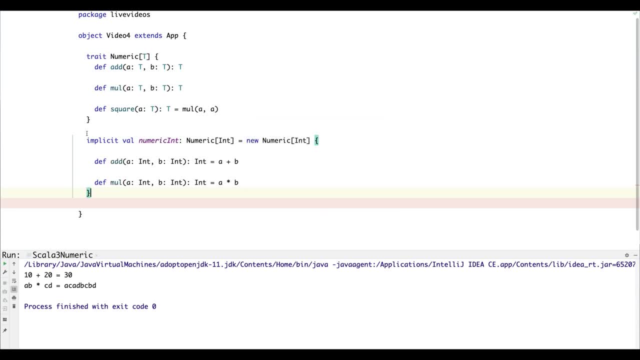 class. so the way we do that is similar but not identical, so we can copy and paste the old version and um. oh, thank you, train. so we just want to change the syntax. we're going to use the given syntax. we no longer have to create an implicit value, and um, the syntax looks like this, so we 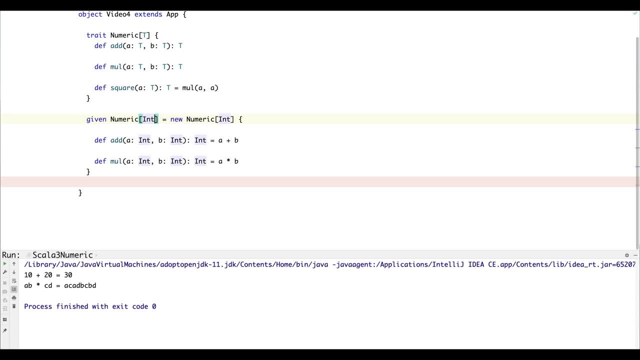 don't need to name this. we can just leave it anonymous and then we use the with keyword and: uh, that's what we need to implement an instance. so, apart from that, everything's the same. we can still go ahead and implement the actual methods in the same way as last time. 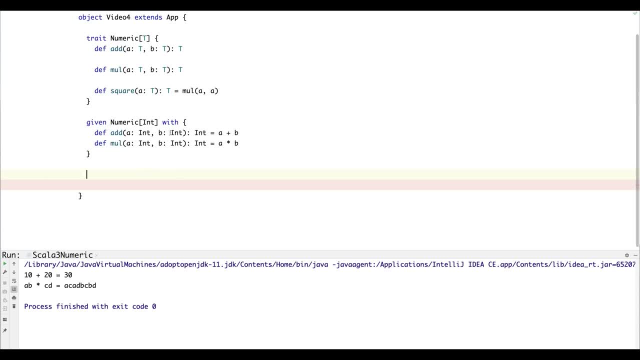 so the main change here with scala 3 is the um, different syntax and um. they got rid of the implicit keyword or you can still use it, but it's deprecated. but now you can use different keywords to represent uh, different, different use cases for the implicit. so in this case, when you want to provide an implicit, you use the given. 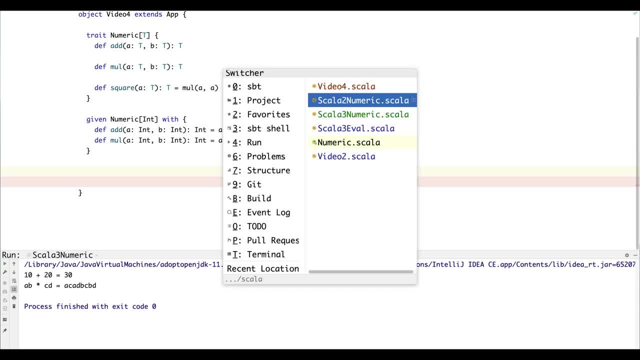 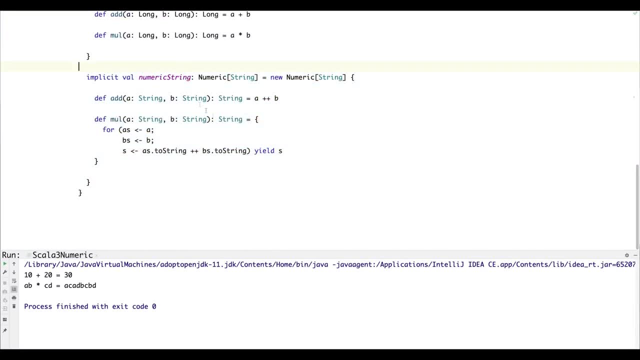 keyword, and when you want to use an implicit, you use the using keyword. so let's just ignore long for this video, but we'll we'll use the uh string instance as well, because i think that's a fun one, uh, even though it's not really practical. it's just. 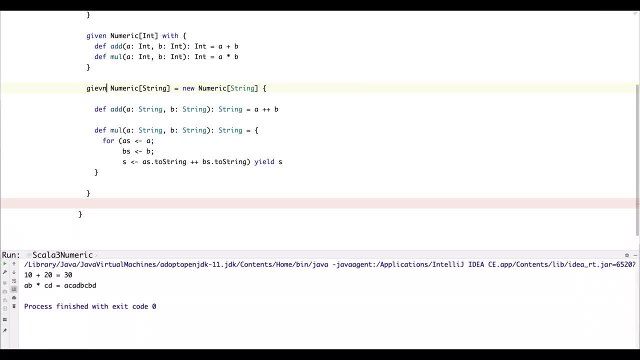 a good example of how you can write an instance for any type t for a particular type class, as long as you can implement the methods in a way that makes sense. so there, we've just converted it to the new syntax, and then we're good to go. 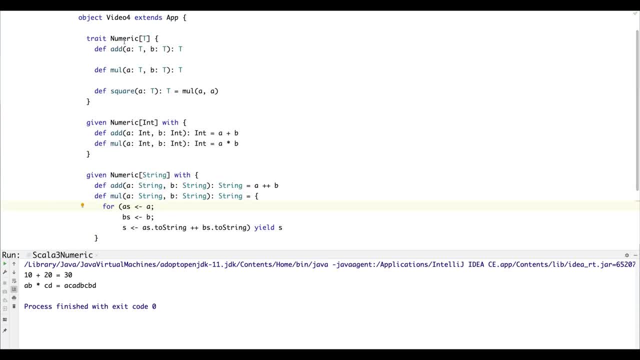 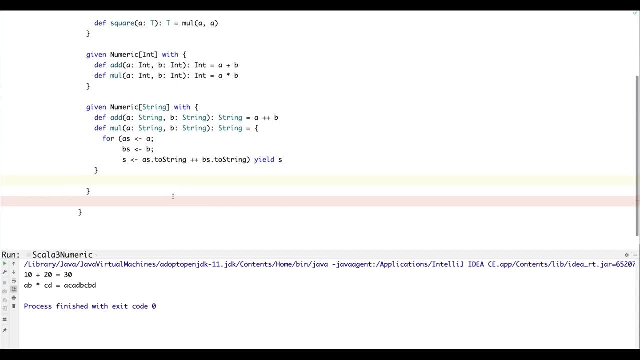 so now we already have a type class- numeric- and we have two instances of the type class. uh, when we want to actually use this thing, we're going to go and we need to summon the thing into existence. so we can use the summon method and we want to bring in an instance of, say, numeric string and then we can call functions on it. 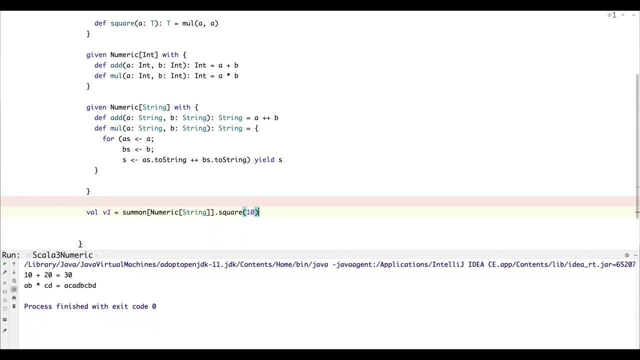 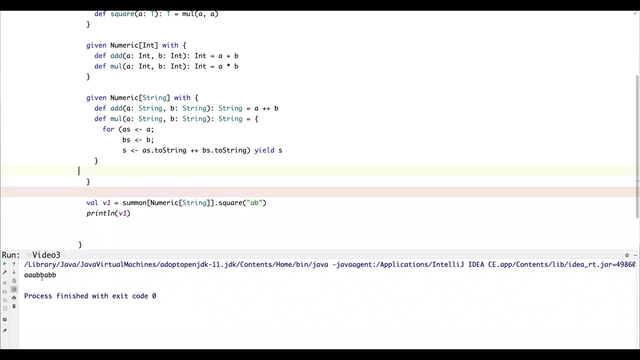 and then let's just square a string like ab and then print the result: um, let's just run that. so we go to compile it. boom, there we go. so we, we multiplied, uh, the string a- b with itself and, uh, that's what the cross product of a- b looks like. so the next thing we 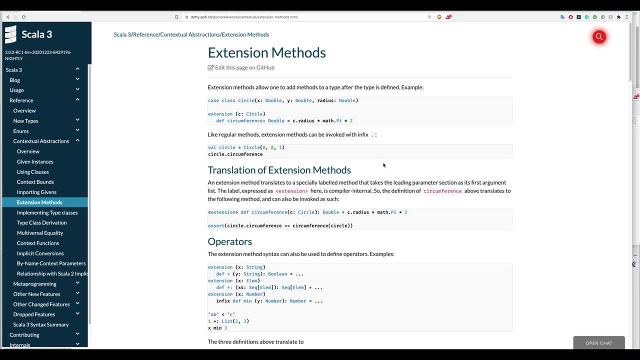 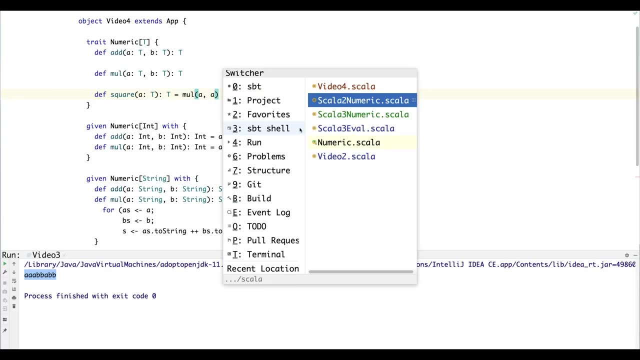 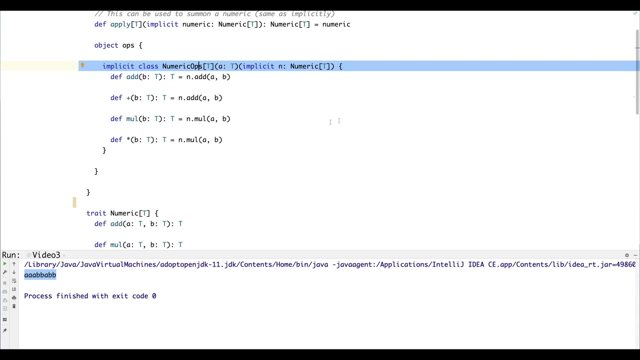 need is a way to add our type class functions as if they were methods on the original object. so if you remember back to the last video, the third video, we used an implicit class conversion. let's take a look at that. so this implicit conversion has to be in scope and it gives us a way to 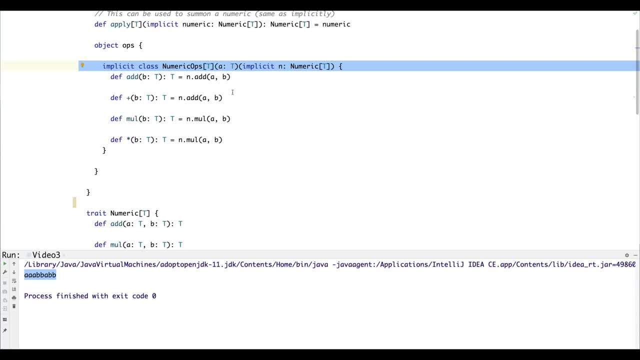 automatically take any instance that has a numeric type in scope and turn it into a numeric ops type, which is essentially a new class that has these operations added onto it. so that's kind of a bit of boilerplate we don't really want to worry about. and that's where extension methods come in. so extension methods are new in scala 3 and they 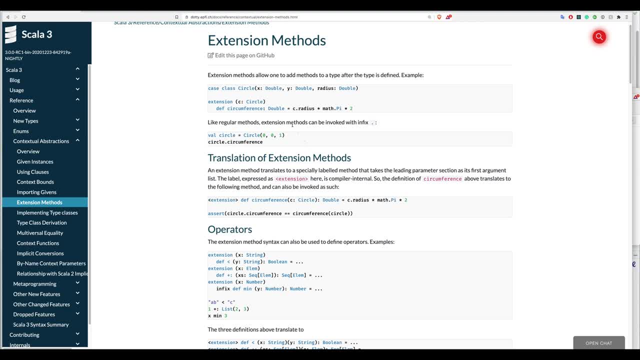 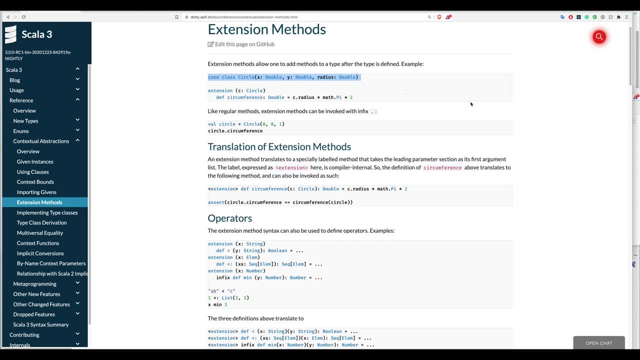 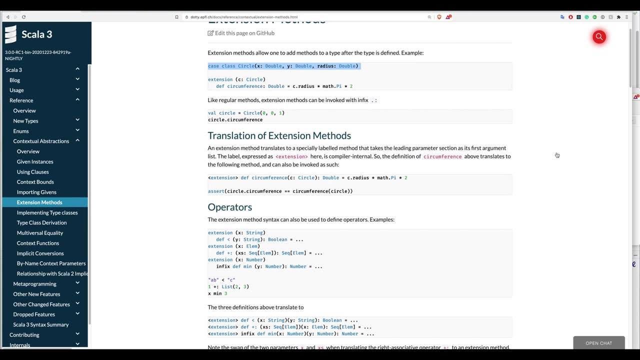 give us a way to take some type and add methods to it. so it doesn't matter here, in this example, it doesn't matter if that type is something type that you don't control. you can always define extensions after the type is defined. so we're going to use that to add a couple. 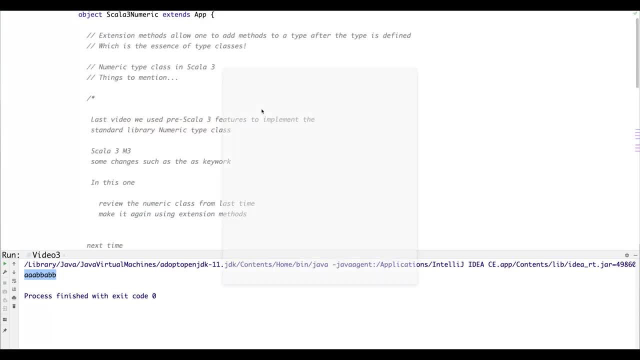 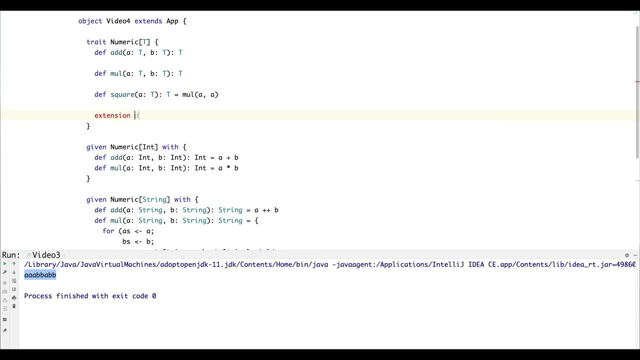 of extension methods to our numeric. so let's do that. so what we want to do is use the extension keyword and then you can create a single. you can create a single function like this: we're going to define the plus operator and we're going to add it to some second thing called b, and then we're 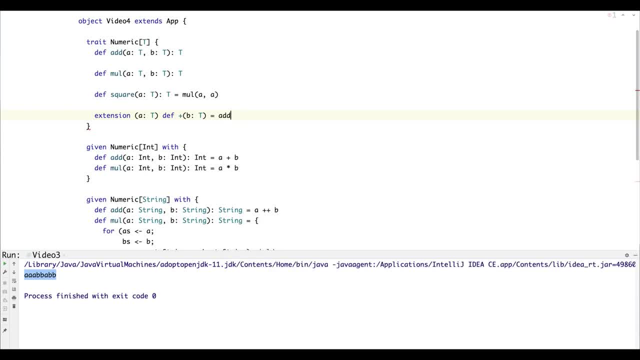 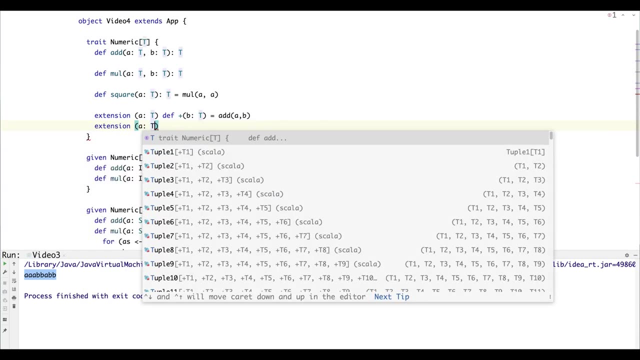 going to define it in terms of the, in terms of add. so that means this is a derived extension method. so it means that instances of numeric don't have to define this. they'll just have it available. and then the next thing we can do is define the. 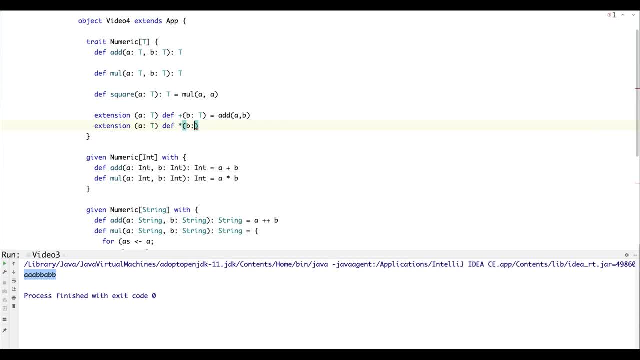 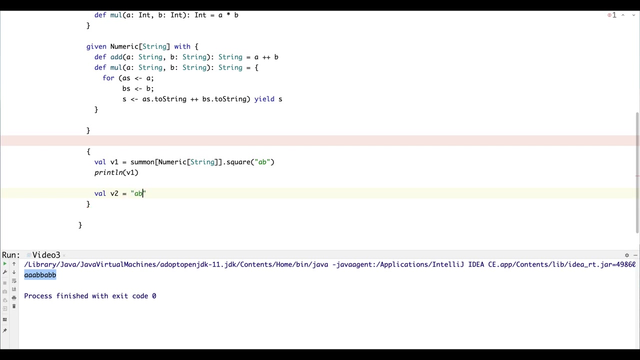 multiply operator and that's just going to call the multiply function. all right, so what that gives us is anything that's in numeric can now use the multiply operator. so let's say we want to multiply two strings. we can take a string like a, b, c, d and multiply it by. 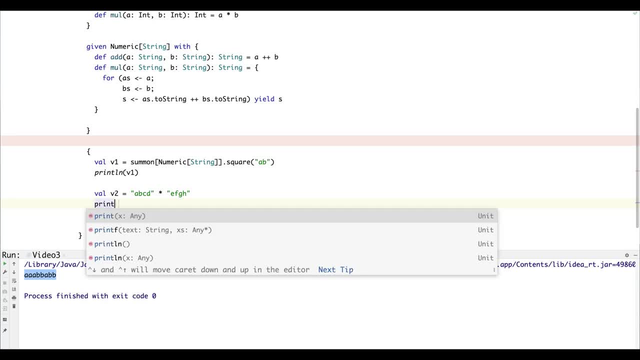 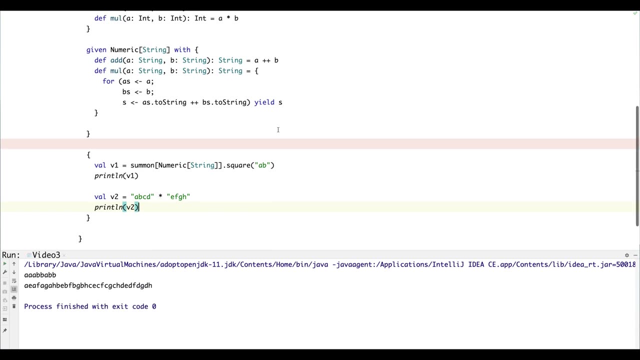 e, f, g, h, and then we can print the result now. we wouldn't have been able to do this if it wasn't for extension methods, because scala had to realize that the multiplication operator was of type numeric. it had to go and find the instance of it. 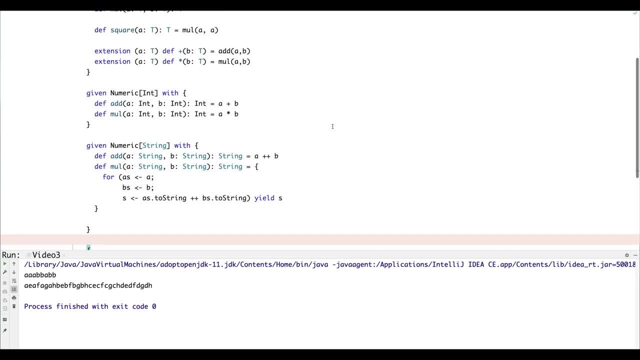 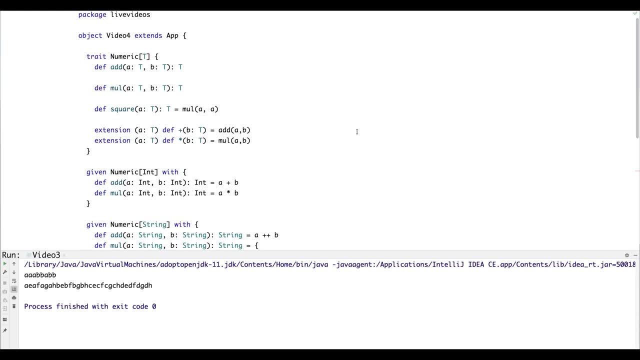 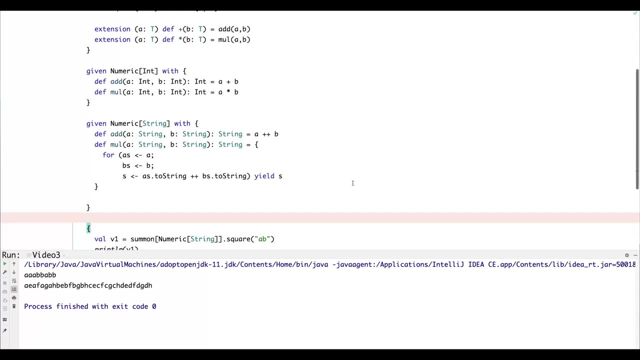 so i think that's pretty neat. it's a lot easier to write type classes and extend them than it was in within scala 2.. there's less boilerplate and the keywords and syntax is a lot more direct. so one other thing we might want to look at is the square function. so let's say we wanted to square a. 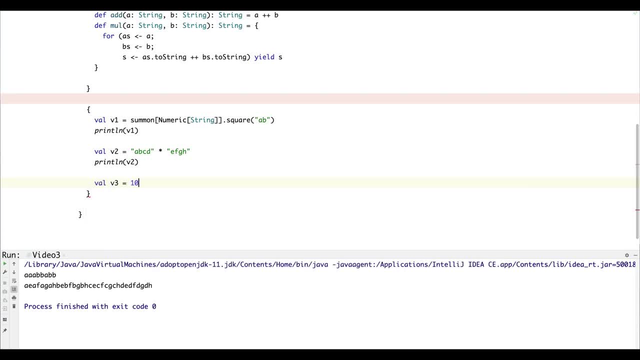 number by kindling double caret, mod �аж. we're gonna print it. you can see that we've got some. we got some red there. it's not happy? um, that's because we can't directly access that, because it's not an extension method, so we're gonna just change that. we're gonna turn square into an extension method. 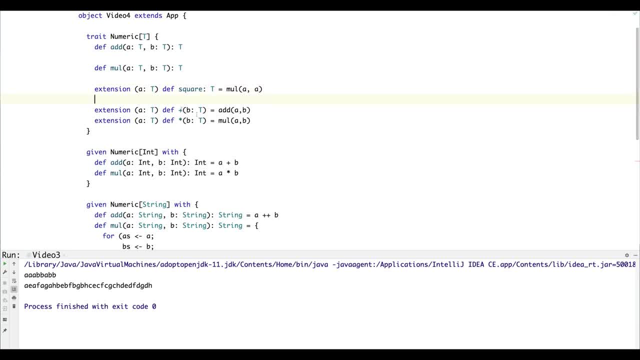 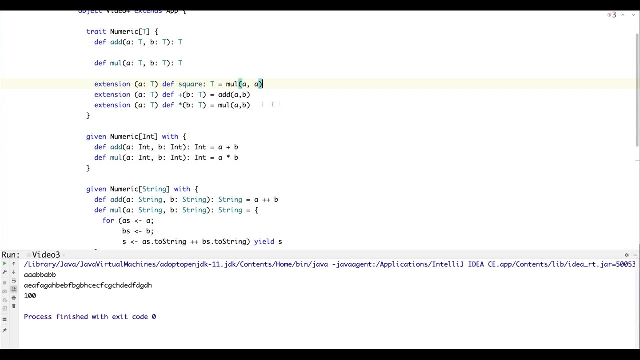 we don't need it to have any arguments. all right, so now we can just call square on anything that's a numeric. i'm going to compile and run. you can see that the square of 10 is 100.. so we can tidy up the syntax a little. there's no need to repeat this extension. 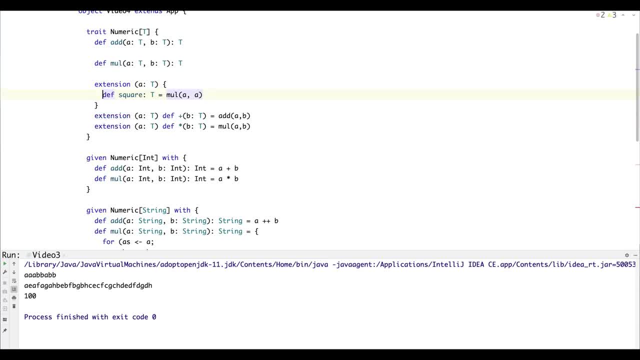 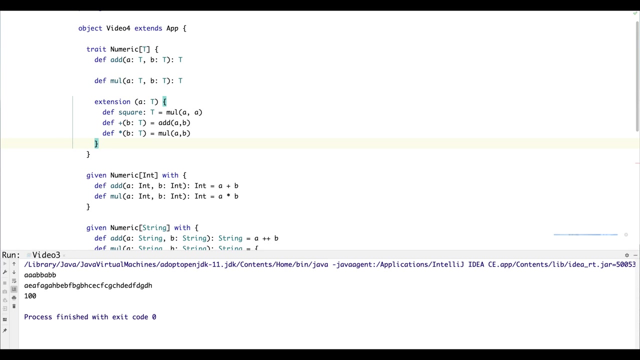 keyword. we can, in fact, put all these things in the same block, so we don't need, uh, this one, we don't need this keyword, and then we can just take these and put them in this block, and that makes things a little simpler as well again. so that's it. it's actually quite simple to build and use type classes using